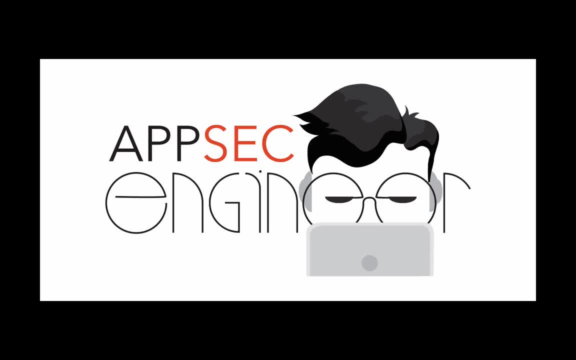 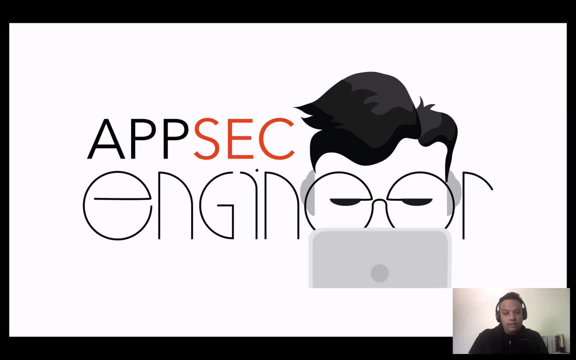 Hi everyone, welcome to AppSecEngineer. I'm creating the series on a regular basis to talk about specific topics in application security. What I'm going to be doing is, in each video, I'm going to be talking about one aspect of application security, hopefully with some demos and some explanations. This week's 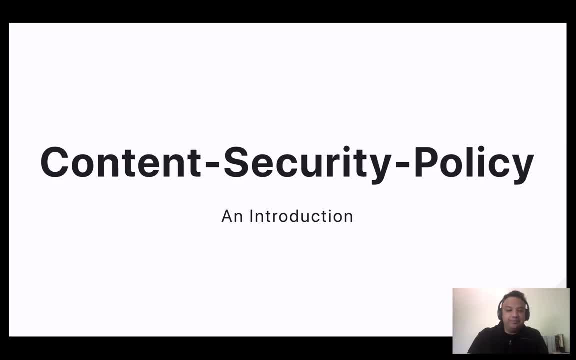 video is content security policy and introduction. Now, in this video, I'm going to be talking about why it's important to have a content security policy. why have a content security policy in the first place? and then I'm going to talk about different ways in which you can implement it, bypass it and, you know, have. 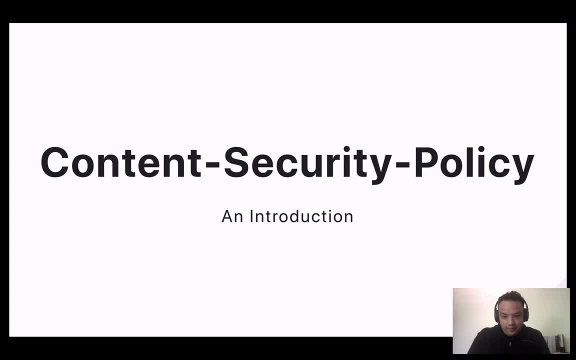 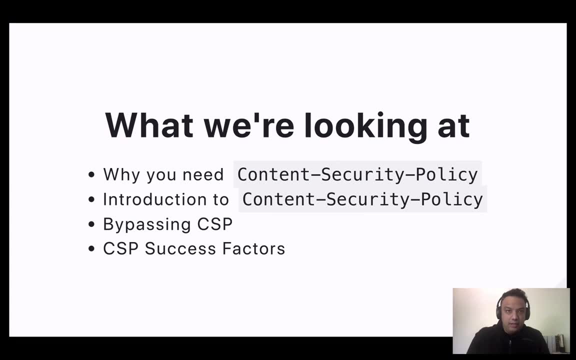 some additional security controls around content security policy. So let's get started. So first of all, I'm going to talk about why you need a content security policy, because that's become one of the fundamental controls for cross-site scripting prevention. So let's talk. 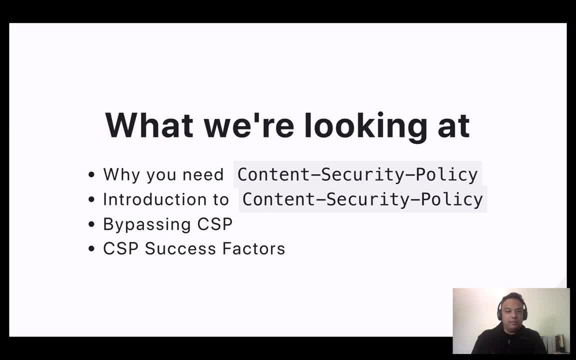 about why you need it, And then I'll be talking about how to implement it. Then we look at some resources in which you can learn to implement content security policy. Then, briefly, I'm going to talk about how you can bypass CSPs. Now, this is going to be especially useful for people who are bug hunting. 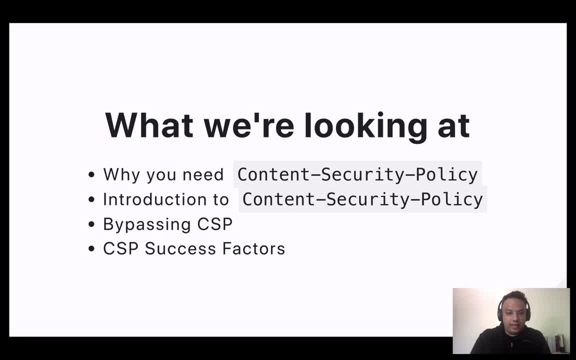 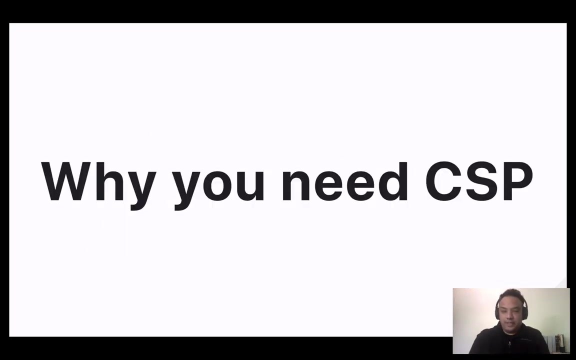 bug bounty hunters or people who are doing pen tests against applications should definitely be looking at some of these factors when testing applications that have CSP. And let's finally look at some additional security controls around CSP itself, beyond the basic CSP controls that it already provides. So let's get started. Why do you need a CSP in the first place? 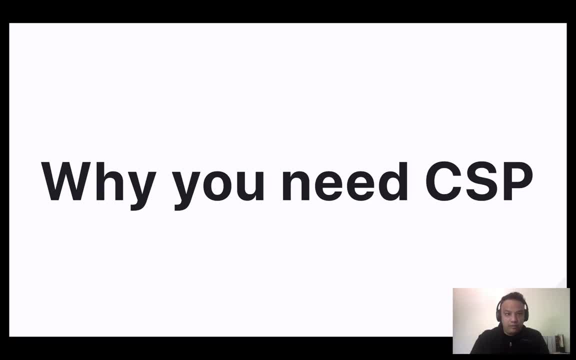 Now, cross-site scripting is pretty hard to prevent. A lot of what happens in cross-site scripting is not something that you have visibility to. It's largely happening on the client side and you don't really have too much visibility of what's happening in terms of the payload, in terms of the attack vector. 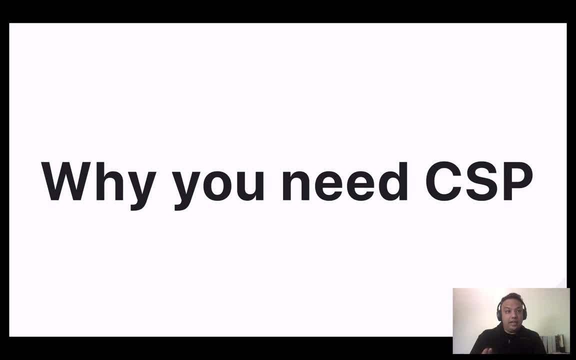 especially with DOM-based cross-site scripting. A lot of this just does not even hit the server. It essentially executes on the client side itself. So that is why, of course, you need a lot of different security controls, And one of the big security controls when we talk about cross-site scripting is input. 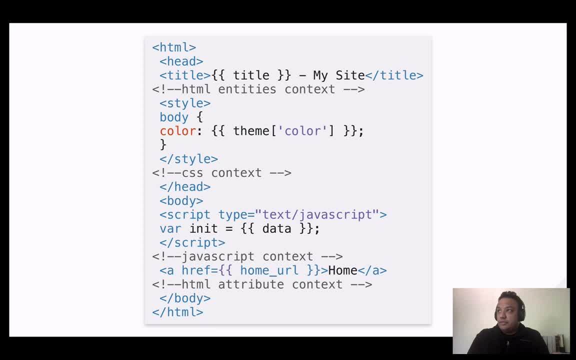 validation and output encoding. However, with cross-site scripting, output encoding is not necessarily the only thing. Now let's look at this example, For instance. here we are loading a template variable to an HTML on the front end. In this case, we have 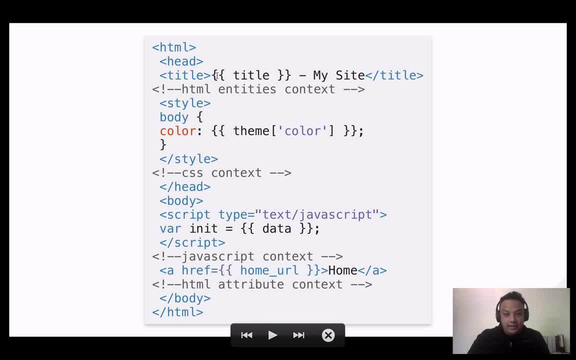 different contexts. So you have the HTML entities context, So you have some template variable being loaded here in the HTML entities context. Then you have a template variable being loaded in a CSS context So you can see that the template variable color of the object theme is being loaded in the 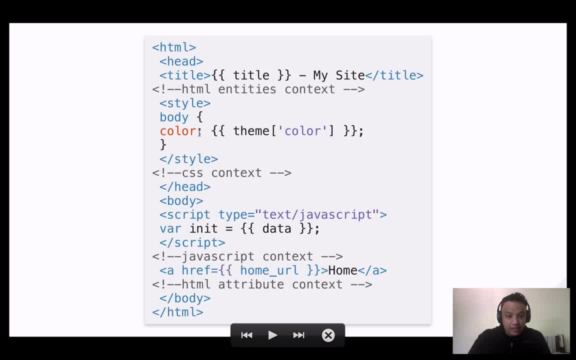 CSS context. You also have the JavaScript context. So, let us say, you load some data from the server side and that is being used to execute some kind of a JavaScript statement That would probably be used in the JavaScript context. And, last but not the least, you also have HTML attributes. So in this, 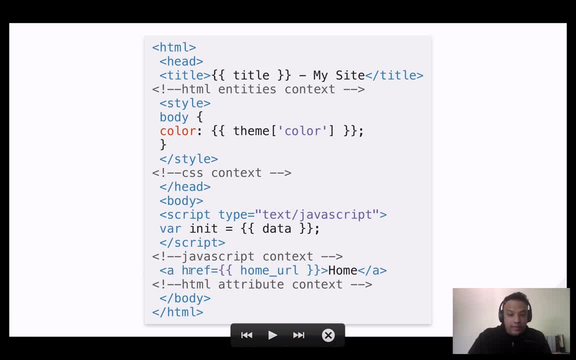 case, we're populating a anchor tag with a particular href attribute, with a particular URL that we're loading from the server side. Now, in any of this, the data that is being easily selected is being loaded in a HTML context based on how the user controls the actual data coming into this particular page, or 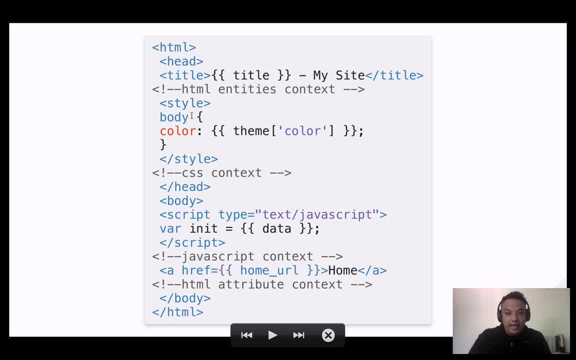 being loaded as part of the templates in this particular page. An attacker can perform a cross-site scripting attack. right, So I can load a cross-site scripting attack here or a cross-site scripting payload were here, here and then, of course, here as well as here. Now, output encoding is a valid defense. 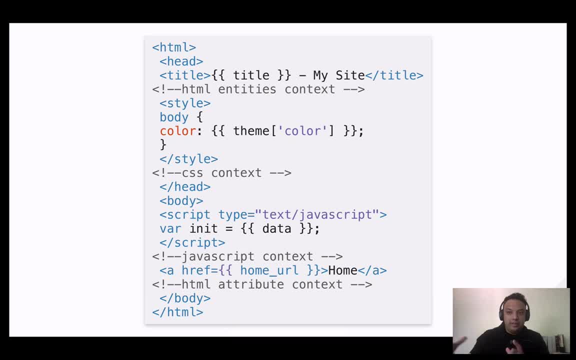 renders the cross-site scripting attack moot simply because it breaks down the payload as data and the browser is not expected to execute data that is being rendered. now, that works usually really well with HTML entities, right? so if you are loading data in an HTML entities context and you're using an auto, 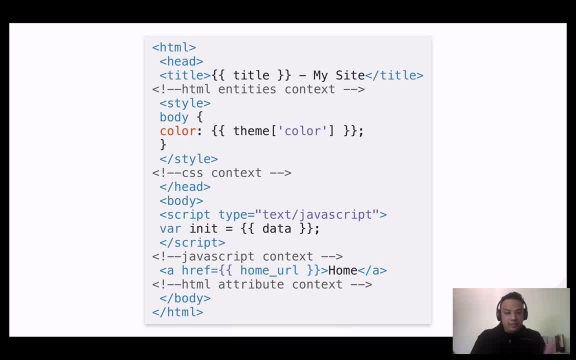 escaping system like Jinja or whatever it is. in this case, I'm using Jinja 2, which is a Python based templating system that auto escapes things for the HTML entities context. however, once you start going into the CSS, JavaScript or the even the HTML attribute category of things, that's when things start to. 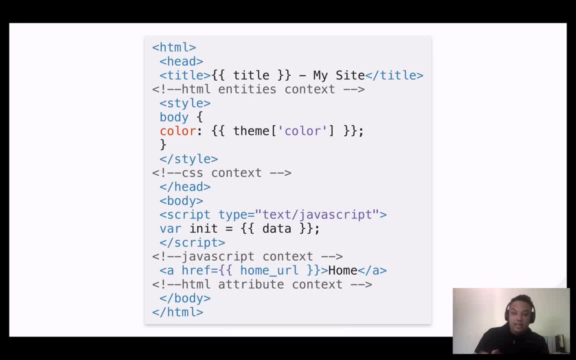 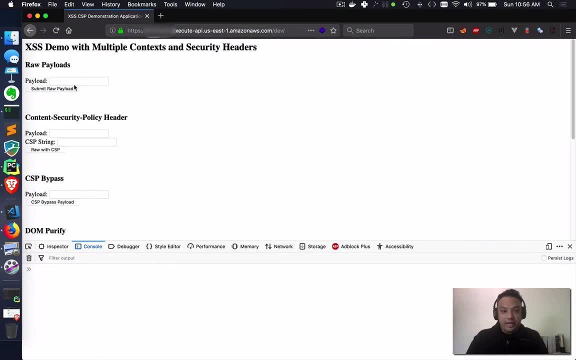 become a little more complicated. for instance, let me show you this example, right? so I have an application that I'm going to load different types of payloads in, and this is a. I'm using a Jinja based templating system in the backend, right? so I'm gonna. 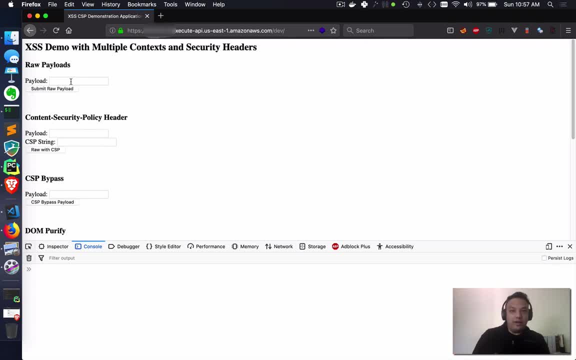 try different types of payloads and some of these payloads are going to be auto escaped by Jinja, right? so let's talk. let's go with a very, very basic payload, right. script alert 1: this is something that all of you would have probably seen when dealing with cross-site scripting: basic payload. right now let's look at. 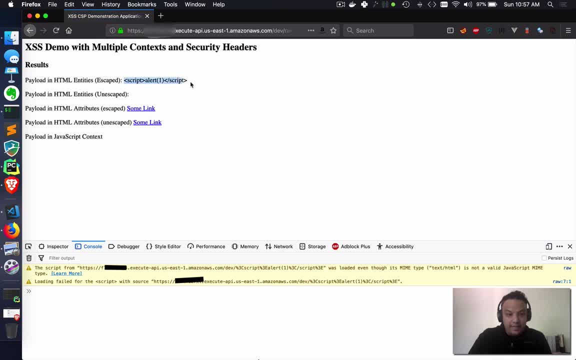 what I've done here. so the first one is the escaped context. this is the HTML and the new看ie context, right, so I'm escaping this. however, the second one is unescaped as a result. it rendered at the payload on screen, right? so it rendered the payload on screen. so let's look at the code as well I'm going to talk about. 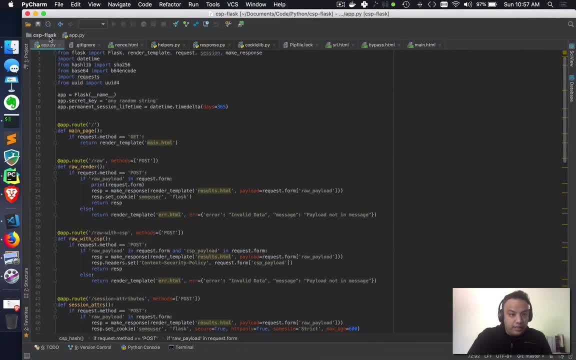 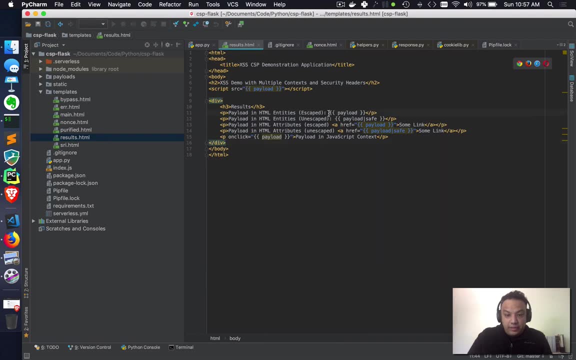 the code a little bit. so, if you look at them, what is coming back? and this is the page in which the results are rendered. I am just loading the Jinja template, which is going to be escaped at this point and, of course, not escaped here. I'm not. 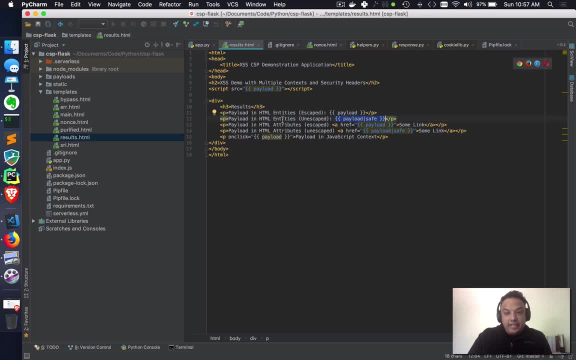 escaped for the fit angels and leaflet in the startup and you'll notice I've not escaped for the face names because this timeframe to поиск файл 여기 HTML entities. now, if I just use Jinja by default, it would automatically escape it and that would be great because I don't need to worry about you know, I don't. 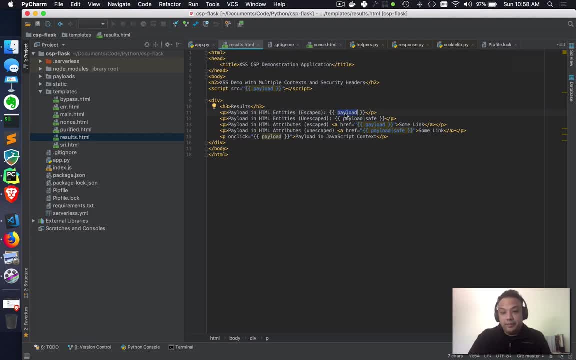 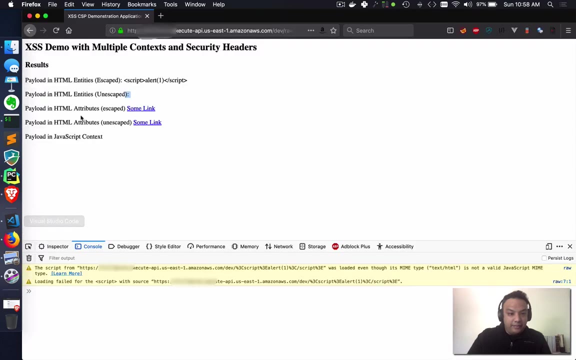 need to worry about contact cross-site scripting simply because the payload is escaped. but the things start getting a little more complicated once I start dealing with HTML attributes and you see that I am still using the auto escape variant here. but let's see what happens in our demo, right? so let's go back and 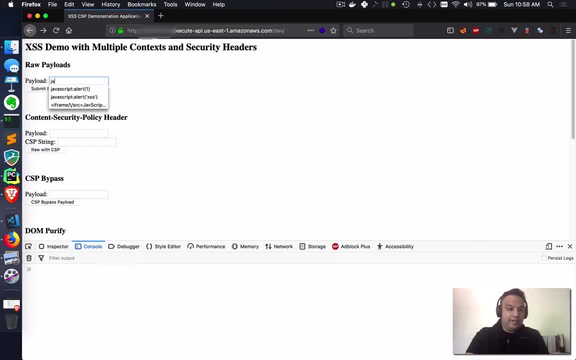 load a different payload, which is JavaScript alert 1. this is the URL style payload that we're using to execute cross-site scripting. hopefully now, as you can see the entities, it does not work simply because it's not loaded as a JavaScript entity. again the same payload does not work, however, if I click even on. 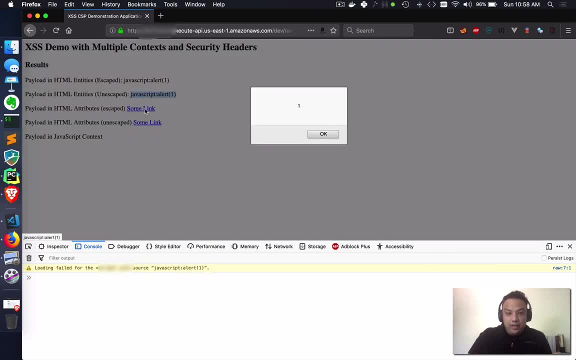 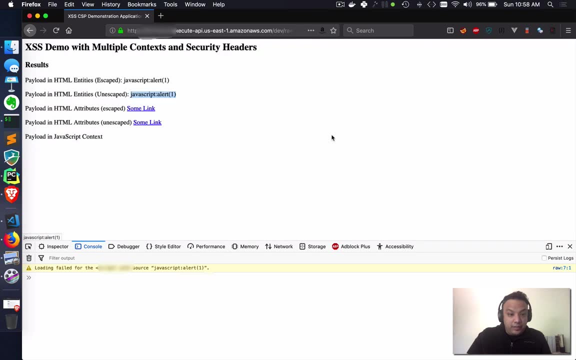 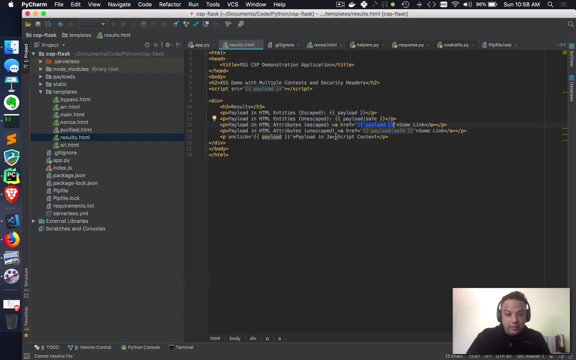 the escaped variant. it renders the payload simply because it is a URL style cross-site scripting that I'm doing here, right, and if you look at this as well, it should render it simply because I am executing this from a JavaScript context. so if you look back to the code, what I'm doing here is I'm saying on: 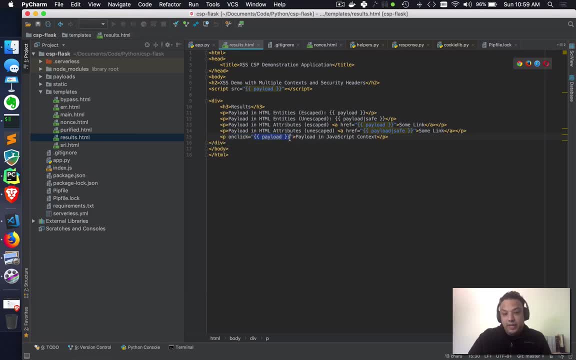 click, render this particular payload. and even though this payload is escaped, even even though I'm using Jinja tool to escape the payload, it's still not good enough, simply because it is executing in a different context. so with HTML entities, things are typically safe, even without our escape templates. however, if 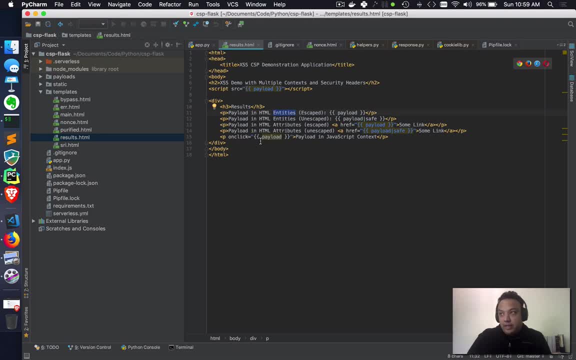 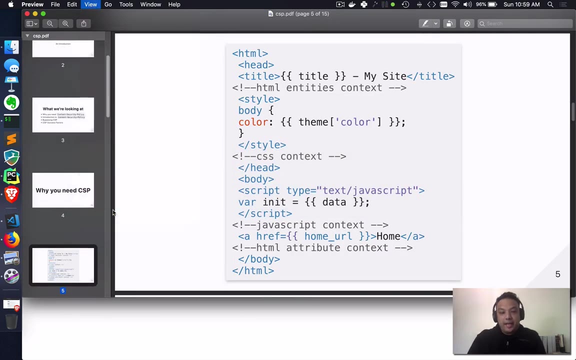 you're loading it in, attributes are in context or CSS context. that is when things could start getting a little more complicated right? this is what I'm doing here. now let's talk about what we are really here to talk about, which is CSP, right? CSP, essentially is, is an. 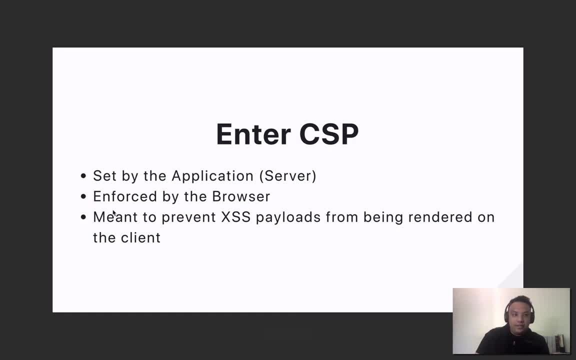 additional security control that the server sets right now. this is meant for the browser to get an instruction to say that hey, browser block this type of attack, so only allow certain things and block things that are not part of the specification. so it's essentially a header that is set by the server, meant. 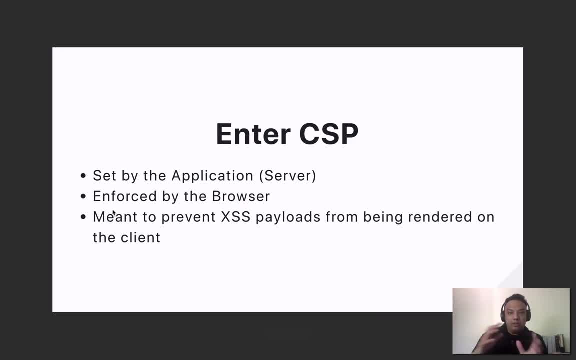 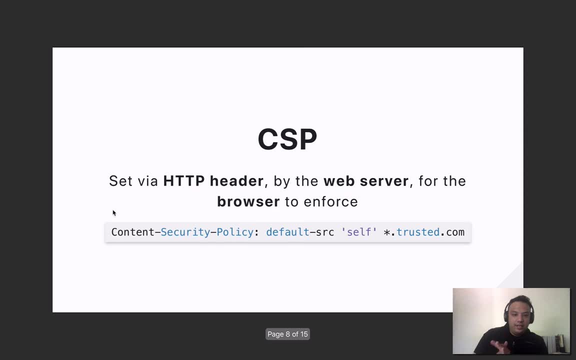 for the browser to actually follow certain rules and discard certain payloads that are outside of the rule set. what you would do with the CSP is something like this: right, so it's an HTTP header set by the server for the browser to enforce, so it would be something like this default source self. 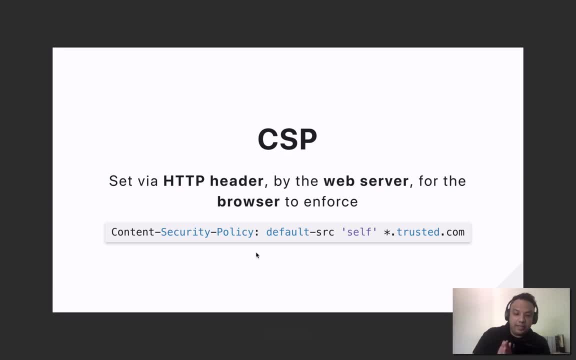 or start our cluster calm. in this case, what would typically happen is that my web server would indicate to the browser we are an HTTP header, that the browser should load client-side code only. well, if it's from self, which is from the same origin server, or from stardot trusted comm. so anything from trusted comm domain would. 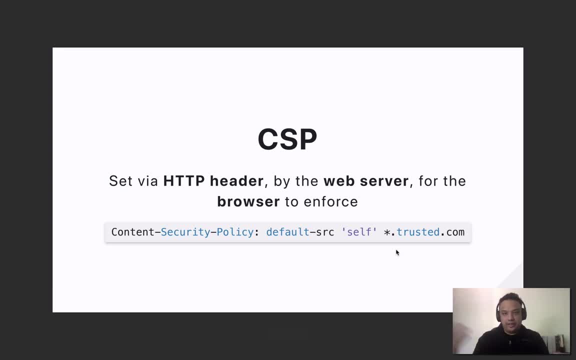 be loaded on the browser. or let us say I'm referencing a JavaScript or the CSS or a style or whatever it is, it would be loaded on that particular DOM, right on the browser DOM. so essentially, this is a header set by the web server for the browser to enforce, so the browser really sees this header. 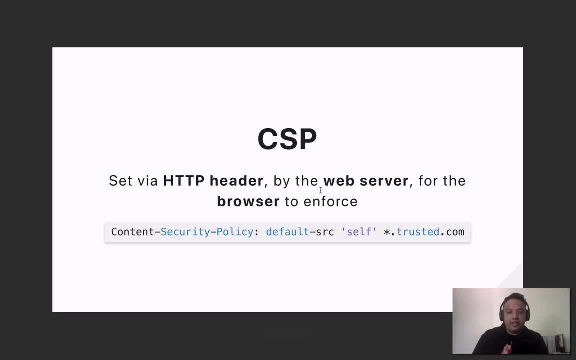 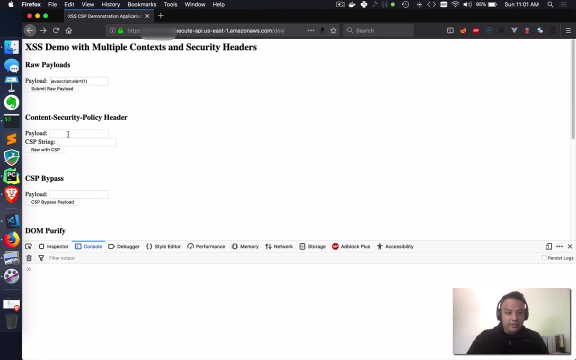 recognizes it as a particular set of instructions, a security instruction- for it to follow, and performs the action accordingly. right now, let's quickly look at a demo of CSP. right? so I'm going to use the same exact example with this, and we'll talk about different types of CSPs and how you can validate. so let's design. 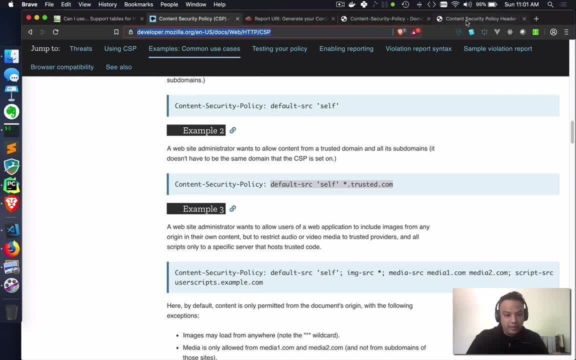 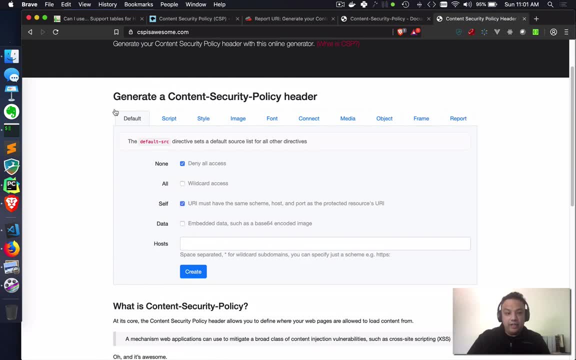 a CSP real quick with a CSP is awesome, calm. so let us say: I want to make sure that we have a self, so the default source is self. now this is very important in a CSP scenario. if you use default source, the idea is that this kind of gives you a single instruction. 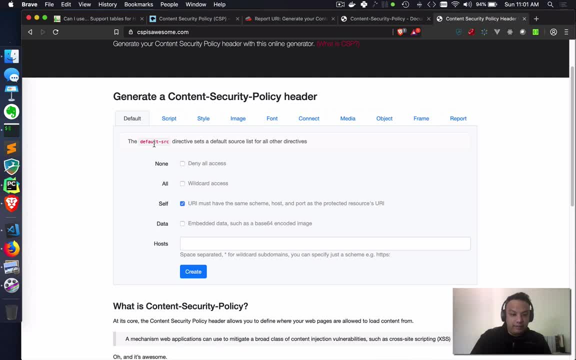 to ensure that all of the content is now only from self. so in this case I'm saying that the default for all possible content types is the original server, which means that anything loaded on that particular DOM will only happen from the same origin server. it will not load, let's say, you. 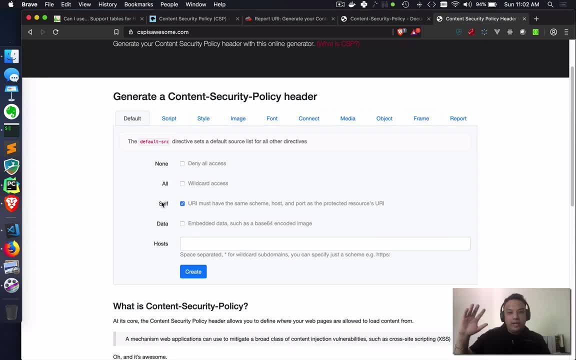 give. let's say you include a script from jQuery, CDN or Amazon or whatever it is, it would not load. it would only come from the same origin server. right now you can, as soon as you do, a default source. typically, what happens is that, unless you want to have specific instructions for other content types, 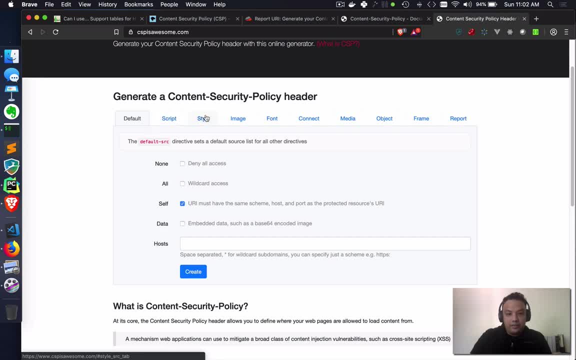 right. so in this case you have default, you have script, your style, your image, your font. now let us say you only want all resources to only load from your default source. it means that you can just go ahead and do default self and you're done with the whole instruction. you. 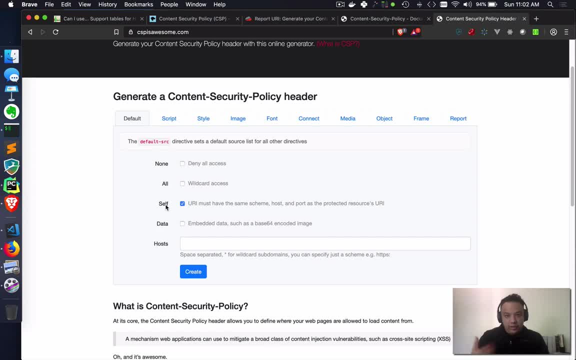 don't need to do anything else, but typically this is not the case. you'll need to have a lot of different sources. so you're probably loading fonts from Google fonts. you're probably loading styles from somewhere else, from a third-party CSS. you're probably learning something else from jQuery. you're. 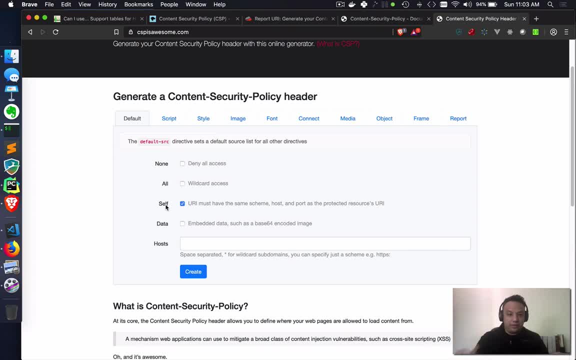 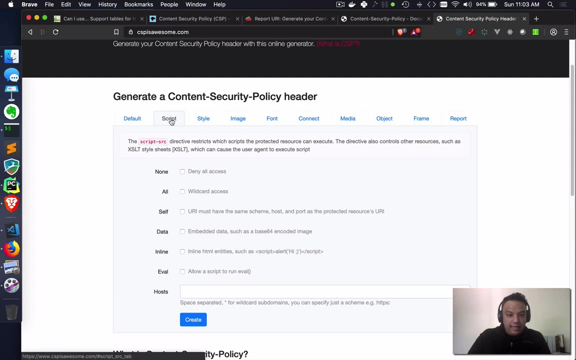 probably learning something from angular or whatever it is. you're loading it from third-party sources, so this may not work for real-world applications, unless you have all of the client-side code being loaded from the same origin server right now. in this case, what I'm going to do is also define that all of the 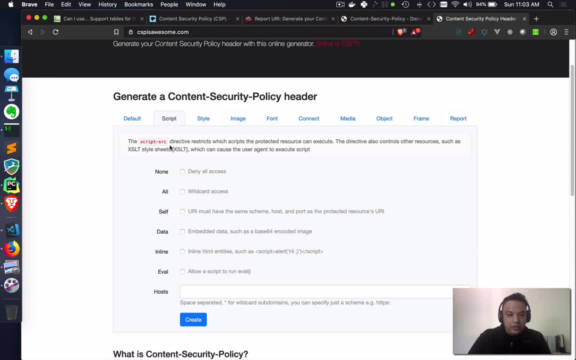 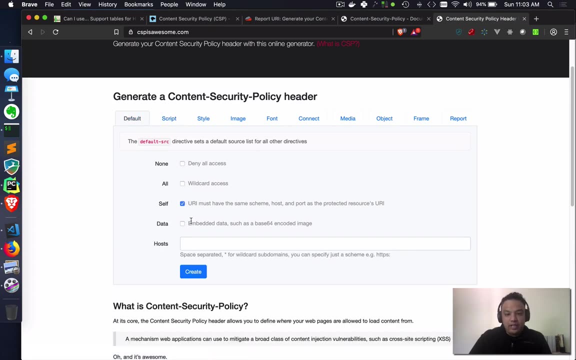 JavaScript- this, the source of all the JavaScript- should be loaded from the same origin server, right? I'm going to load all of the JavaScript from the same origin server and I'm also going to specify that the default is the same origin server. so let's just set this and it would generate a nice little content. 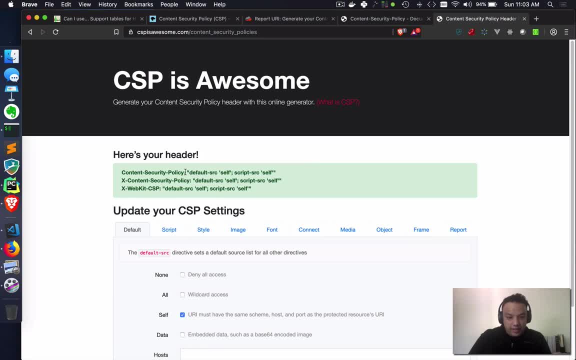 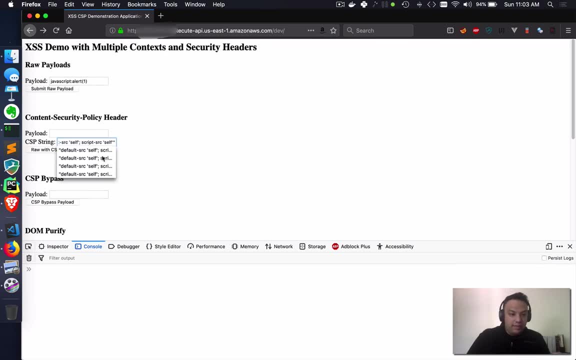 security policy header for us and I'm going to use this header in my screen. so let's just quickly go to my demo app and say this: right? so I'm going to load that the default source is self and the script source is also self. now let us. 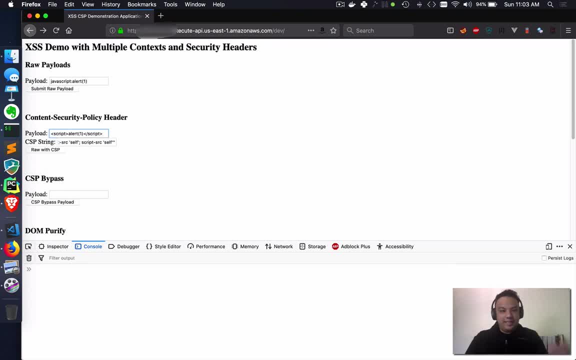 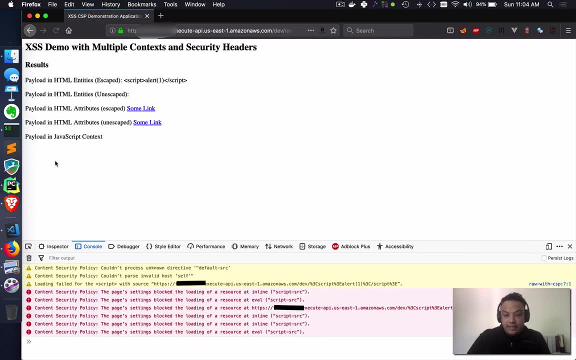 say: I go ahead and run this payload. this is the same exact payload that I ran the previous time. hopefully we should see that it does not execute and you see that it did not execute, right. so it said that the page setting, you can see the console, the JavaScript console, here. 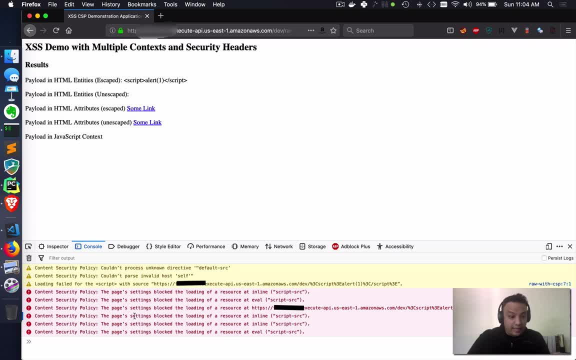 essentially coming up with a bunch of warning, saying warnings and errors. of course it says that you know what content security policy prevented the load of this particular inline script. so I loaded a script inline which was script alert, one which it disabled simply because the inline script was not allowed, eval was not allowed. so one of the things we saw 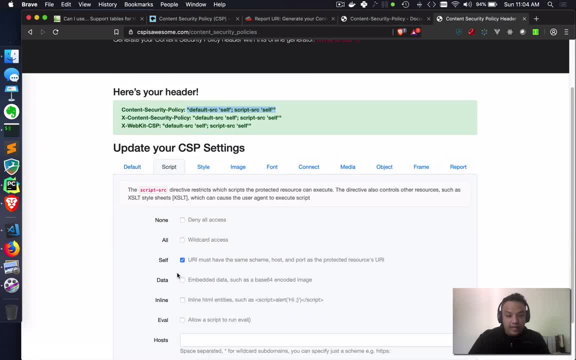 here was when you were setting the script. we did not allow the inline HTML entities. we did not allow the script to run an eval function in JavaScript, so that's why it essentially blocked all of the execution possibilities in that script, which is great right now, even if you have a potentially vulnerable app. 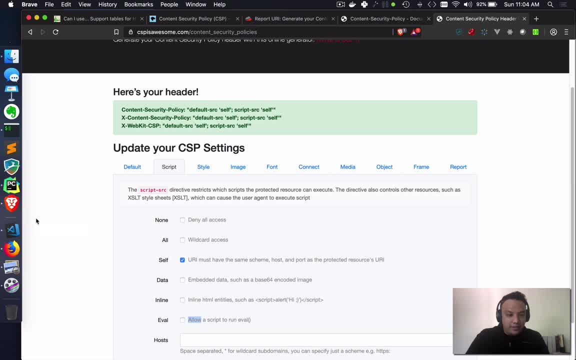 that may be vulnerable to cross-site scripting because of various reasons. a CSP header would essentially prevent or reduce the blast radius of that. it may not prevent all the time, depending upon how the attack plays out, but it may definitely reduce the blast radius of that particular attack. now let's look at another example, right the same. let's use 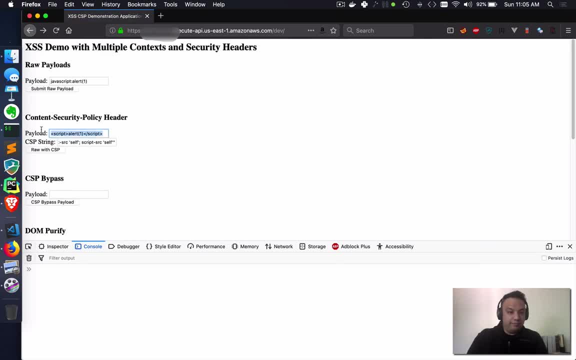 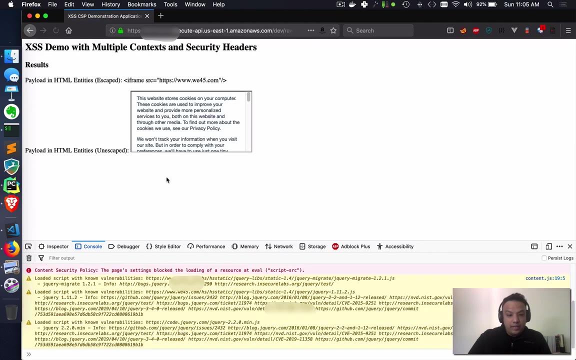 the same CSP. however, this time let's go with an iframe right. so I'm gonna go with an iframe that links to we45.com and you'll see, this time it executes the iframe right, because what what we have done is we have not specifically mentioned or we have not specifically 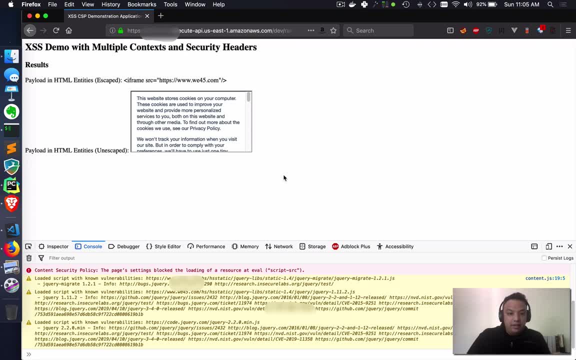 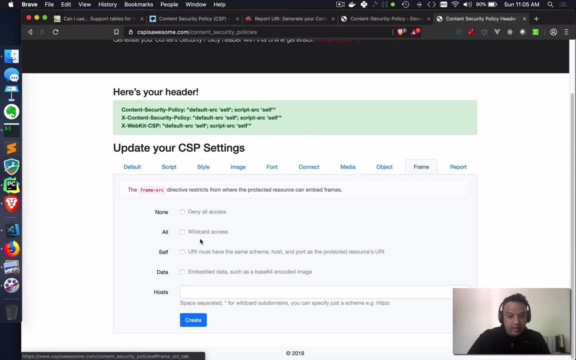 set the CSP directive to not include iframes right. as a result, it now loads iframes right. so let's quickly look at how we can do that. let's go back to our CSP is awesome. go to frames and say: no frames, I don't want to load any iframes. 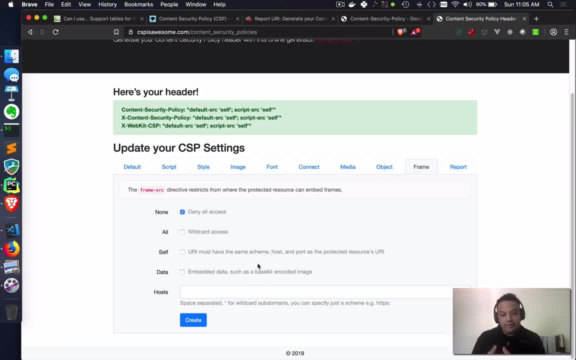 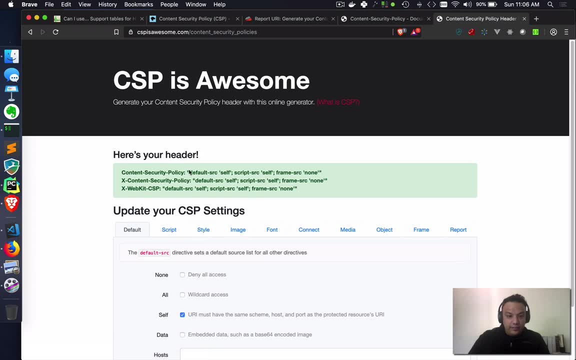 at all, because my website or my application does not require iframes. it's never needs any iframes. so let's assume that that's the case. and now I go ahead and say this, it will generate a different header. so in this case I'm saying default source itself, script source itself, but frame impossible. 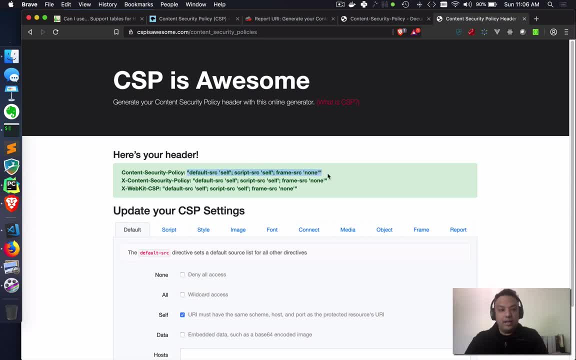 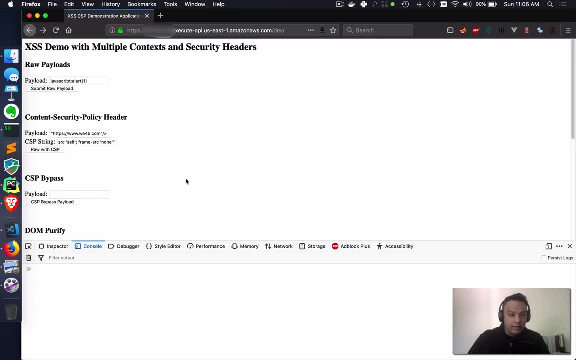 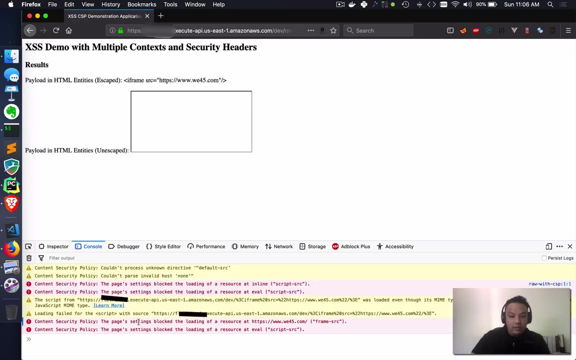 nobody can set any iframes on this. it's not possible because I don't need iframes. now let's go ahead and try the same exact payload out and use the same iframe directive and you can see that it did not load, so blocked the load of this particular iframe. 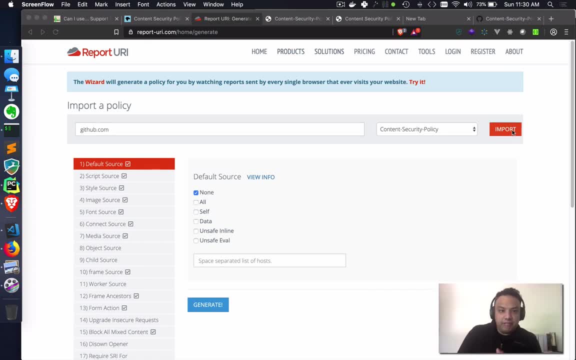 right now. let's look at the CSP of a very popular website out there. now let's look at githubcom's content security policy. now, if I import it, what it's going to do is it's going to give me the CSP. so I'm using the report-uricom. 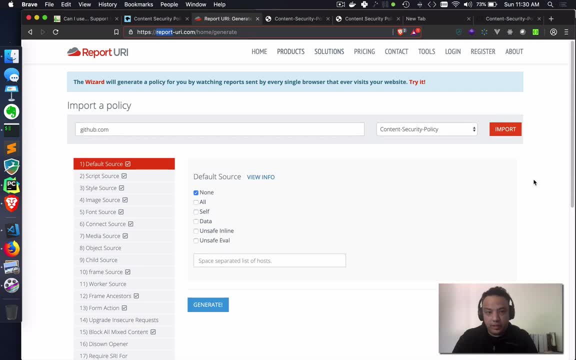 to which is a security site which allows you to set and validate and look at violations of your CSP as well. now this site also has a policy importer. when I'm using its policy importer to see what kind of a policy does a site like github or Google have right? so in this case, github, one of the most popular sites on 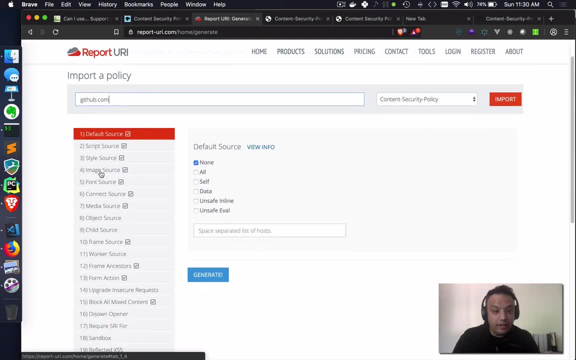 earth has a pretty granular policy, as you can see. the first thing you'll see is that the default source is set to none. now, this essentially means that deny all access. right, so the default source set to none means deny all access. however, obviously, github loads stuff from different resources, doesn't just? 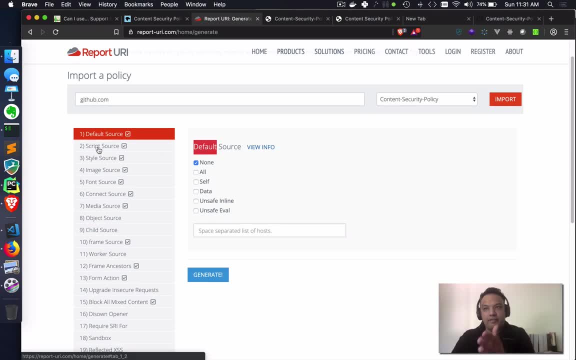 mean that they don't load anything on the site. it clearly means that there are very granular, specific directives that github is loading as part of its content security policy. so you can see that it's loading script source only from github- github assetscom, style from github- github- assetscom, and it's also allowing 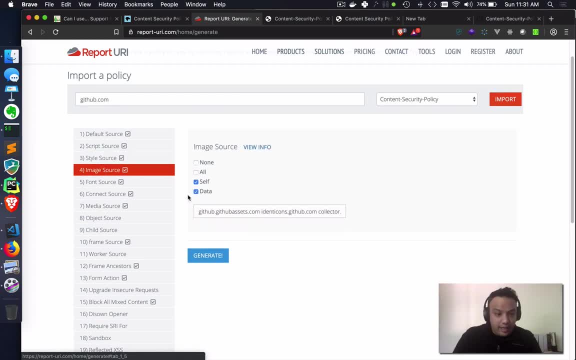 unsafe inline. they probably have a good reason for that. image is from self as well as some data. so let us say you want to load some base 64 encoded images, you can do that, and from these specific sources as well. so you can see that github has very specific granular instructions and all of this. 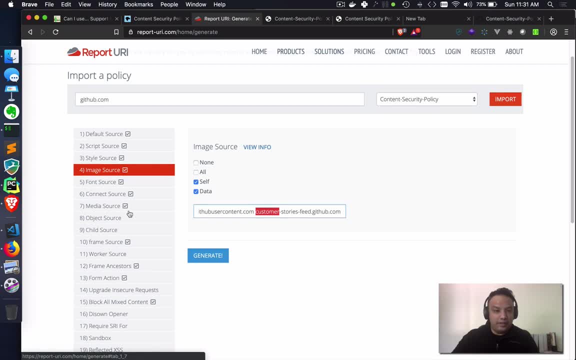 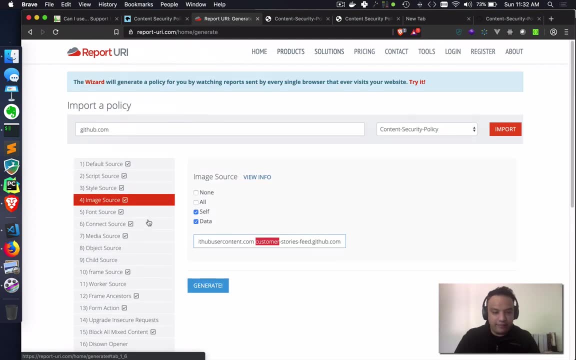 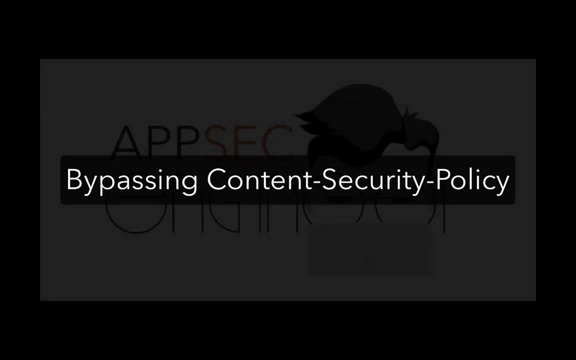 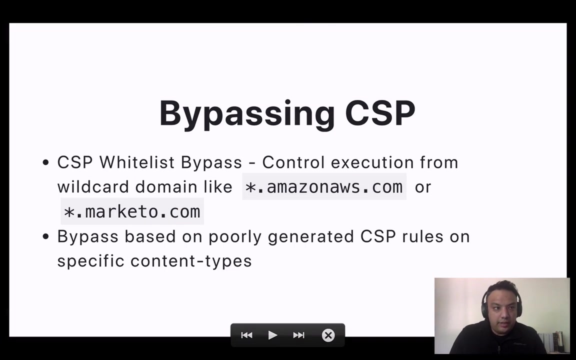 that is under the checkbox means that github has specified all of these elements as part of its CSP, and you can see the frame ancestors, mixed content, so on and so forth. a lot of stuff is being rendered as part of githubs content security policy. let's look at a very popular type of attack against CSP, which is CSP. 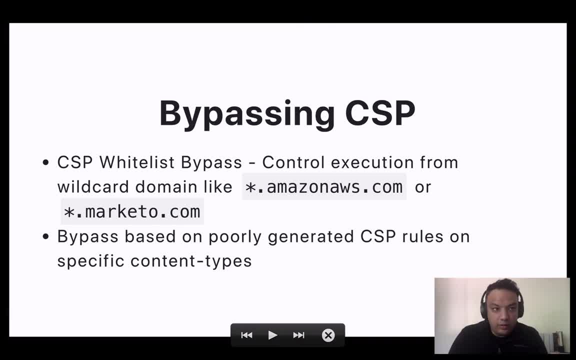 whitelisting bypass. now, one of the things you can do with a content security policy is set up wildcard entries or domains. right now, let's say that I have an application that is loading JavaScript from a particular s3 AWS s3 bucket. right, there's a very common pattern where you have static 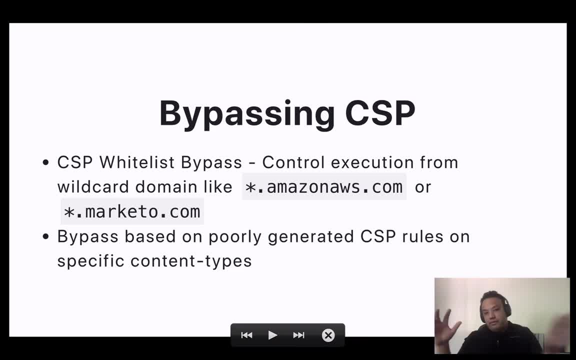 assets stored in a AWS s3 and you have JavaScript, CSS, images, fonts loaded from that particular s3 bucket or from some third-party site like marketo for analytics and so on and so forth. right now, this is a very popular way of doing things and a lot of 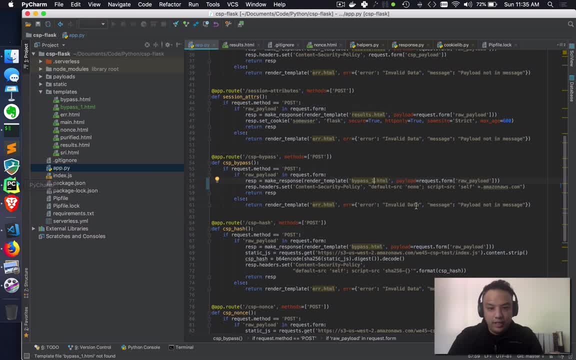 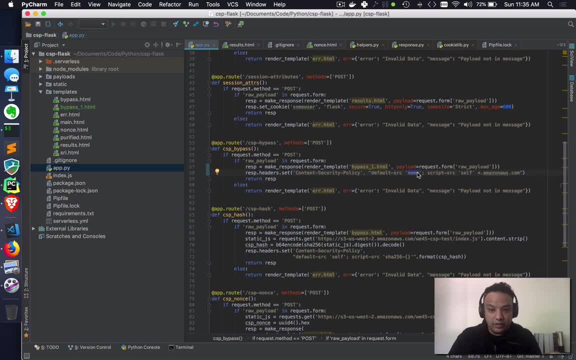 developers do something like this. now let's quickly look at the code. so in this case, what I'm doing is I am setting a content security policy with a default source of none, which is a good thing. I'm blocking all access, but then, in my script source as setting up a 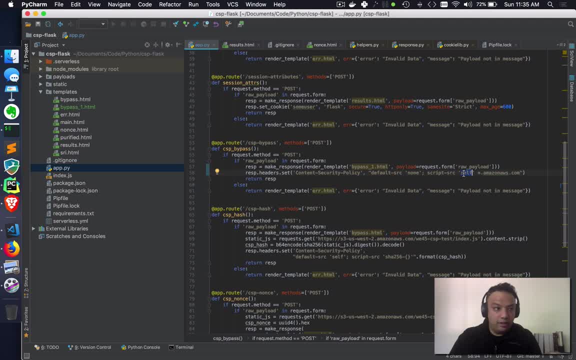 construction saying that you can load JavaScript from self, or you can load if the script source is star dot Amazon, AWS, comm. now you can probably see where I'm going with this. first of all, if an attacker is able to find that your application is vulnerable to cross-site scripting and the attacker sees your CSP, 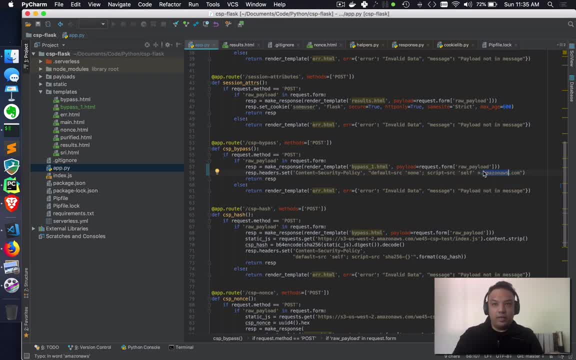 to be set to this wildcard entry. all the attacker would now have to do is set up another s3 bucket, load some malicious javascript resources in his or her own s3 bucket and then start using that to perform cross-site scripting against your application. right? so let us say you have. 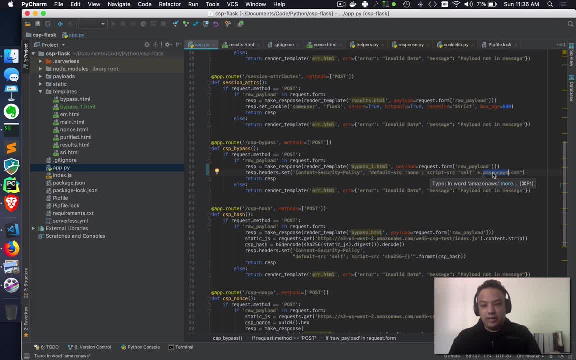 genuine site dot s3 dot Amazon AWS comm and you're loading JavaScript from there and attacker has evil site dot s3 dot Amazon AWS comm. you can actually. the attacker is now able to load all those resources on your application simply because you have set a pretty large wildcard. 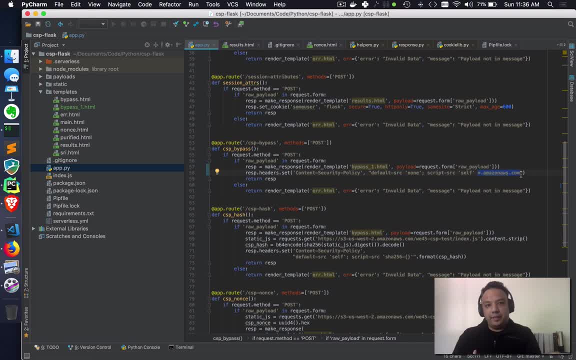 against your application. so if you are someone who spent testing applications or doing bounty hunting or your auditing applications, one of the things that you should look for- especially when you're doing CSP validation or looking for cross-site scripting- is look at the type of CSP that is being set up, whether it 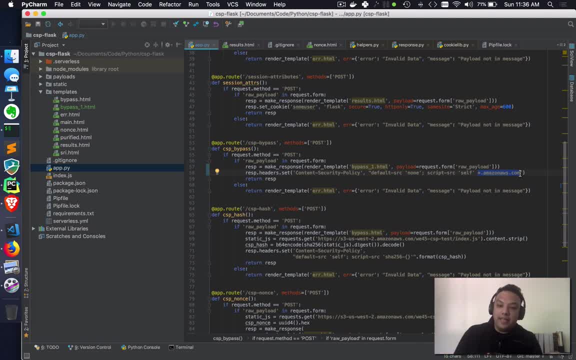 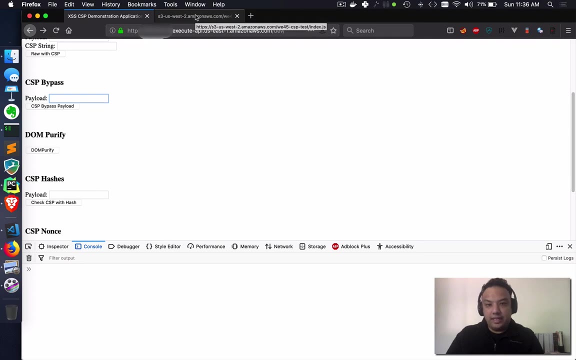 has a lot of wildcard entries and whether the domains of those wildcard entries can be, you know you can influence or control the aspects of the domains of those wildcard entries. now let's take that in a real world example. right now here I have set up an s3 bucket, which is we 45 CSP test. 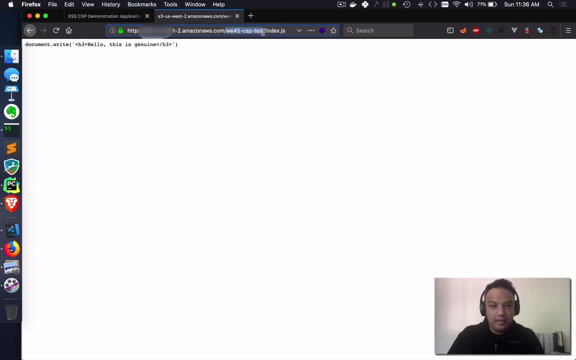 indexjs, right. so I have a particular s3 bucket which has an indexjs and this has the content document on right. hello, this is genuine. I obviously want to load this in my application. so let's say, I take this and I paste it in here now. 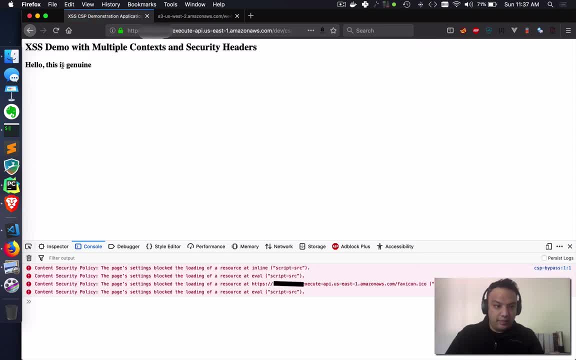 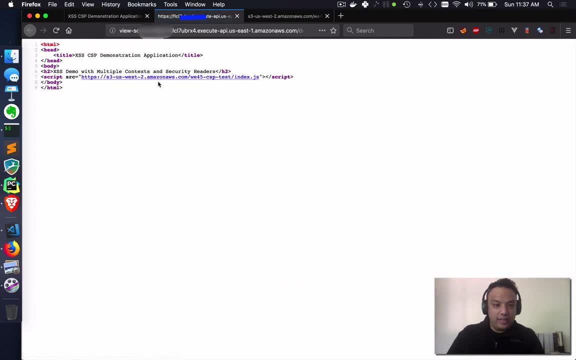 what it's going to do is hopefully load that resource so you can see that it prints: hello, this is genuine, and if you look at the page source, it's script source is set to the source at which I specify that particular script source. now let's take a slightly different example. let's 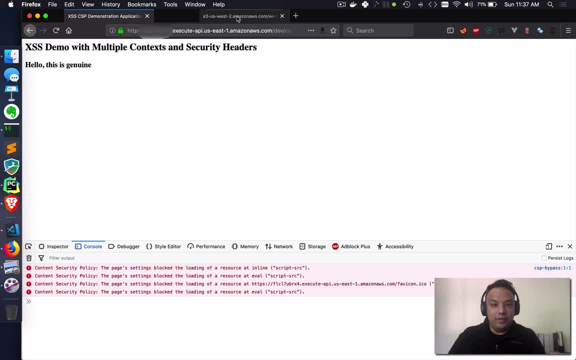 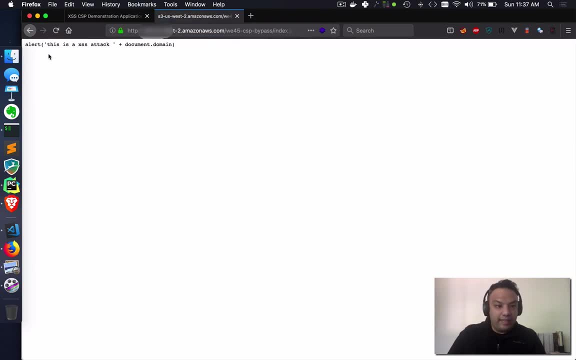 say, attackers identify that you are using star dot, Amazon, awscom. now what the attacker could do is set up a malicious payload like this. so in this case, I've set up a malicious payload with an alert. this is an excesses attack document or domain whatever. so I've set up a malicious payload like this. so in this case, I've set up a malicious payload with an alert. this is an excesses attack document or domain whatever. 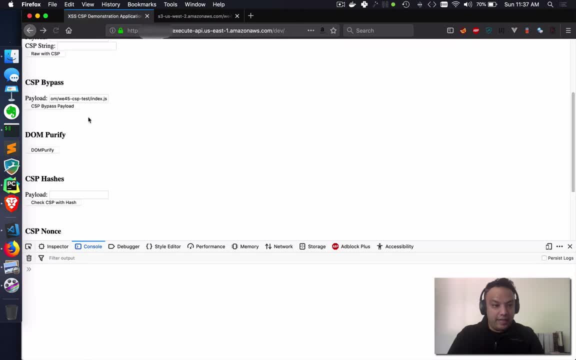 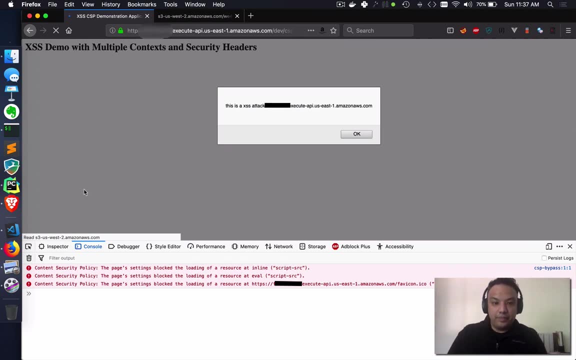 so I'm going to copy this and paste it in to my application and now it should still work, simply because I am loading this particular resource and since I have whitelisted the entire Amazon awscom as a CSP whitelist, this is going to become a huge challenge and attackers will be able to use this and if my 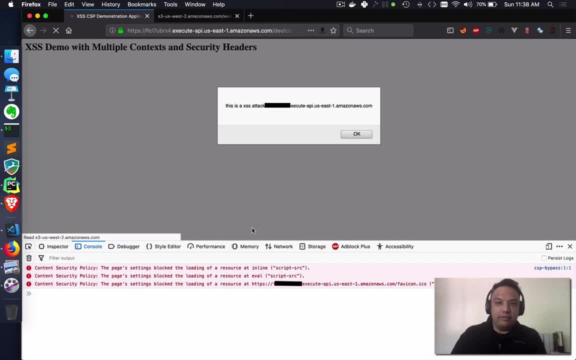 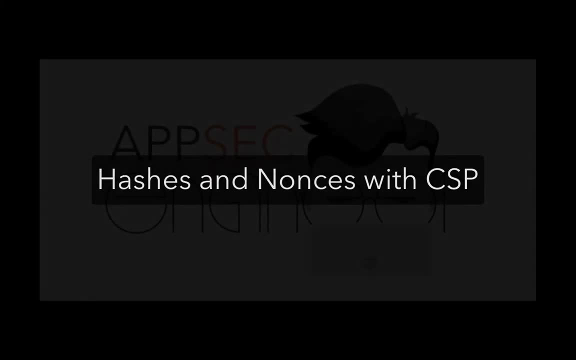 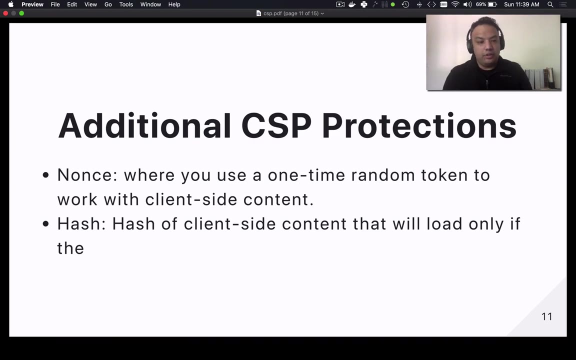 application has or is already vulnerable to some kind of client-side injection. I'm going to take this and I'm going to use this to protect the content security. some of the additional ways to protect with content security policies is to use nonces or hashes. right now, nonces and hashes are additional protections beyond. 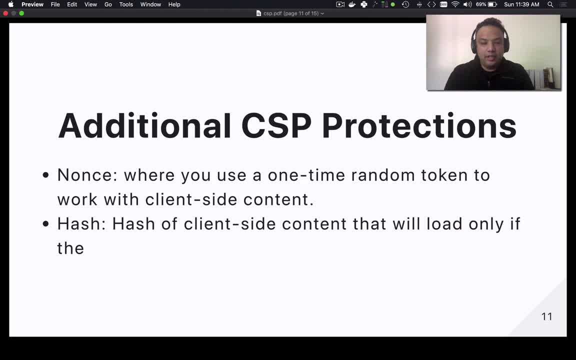 the realm of just the traditional content security policy. so I could use a content security policy with the nonce to say that hey, only load a script that has this particular one-time random token that is also loaded on the client-side. so if your script has this nonce called XYZ and your content 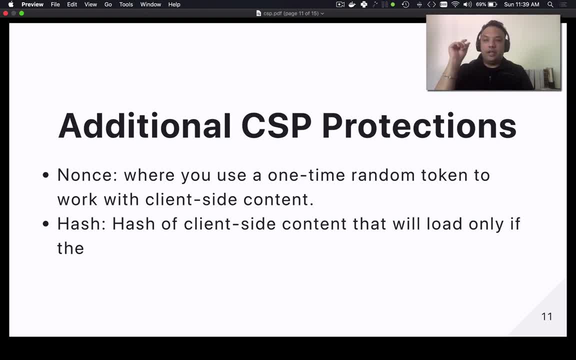 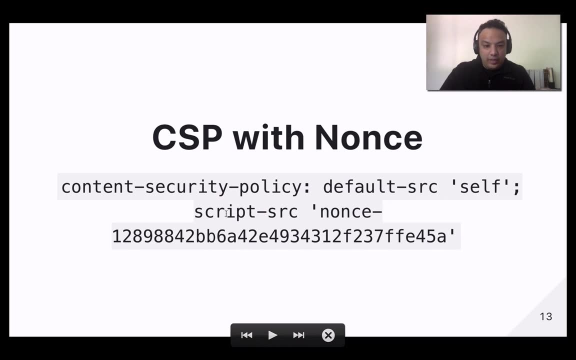 security policy has a directive to say that load only scripts with the nonce XYZ, then that particular script is the only one that is going to be loaded on your application. so let's quickly look at a demo of how this would work. right, let's so. in this case, I have a content security policy loaded with a script. 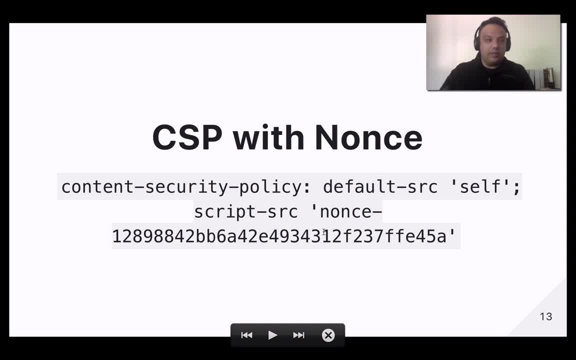 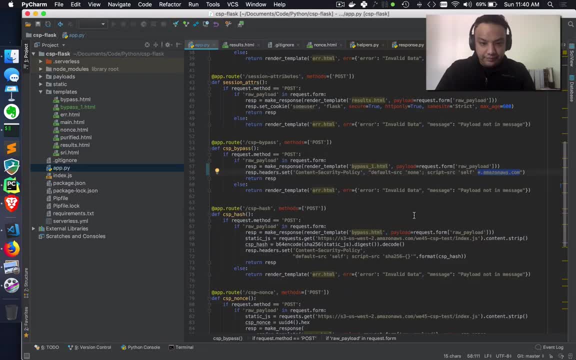 source that says anything that has this particular nonce is the only thing that I will allow to load on that application. so let's look at the code and see how it works. so in this case, what I'm doing is that I am taking the previous example, so you saw. 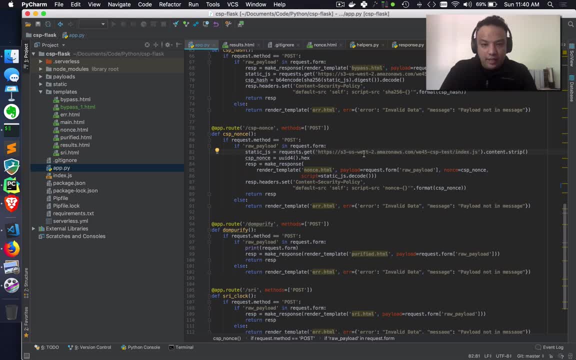 the document, dot write: this is genuine payload. right now, what I'm doing is I am generating a nonce. now, remember, nonce must be a one-time use token only. so every time a page refreshes or the user moves on to another page or moves on through your application, you need to. 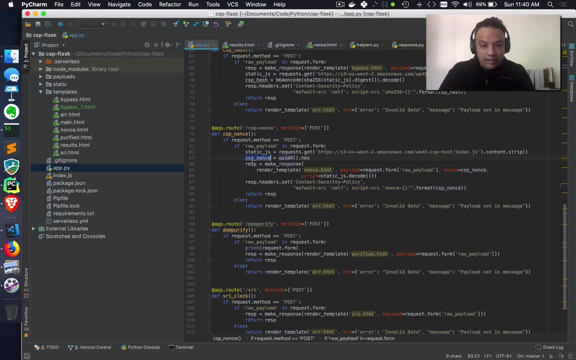 write different nonces, right? so nonce, in this case, I'm just using you uid for and getting the hex value of that and using that as the nonce. right now, whenever I load content, I am going to load it with this particular nonce and I'm going to load that script with that particular nonce. so in this case, what? 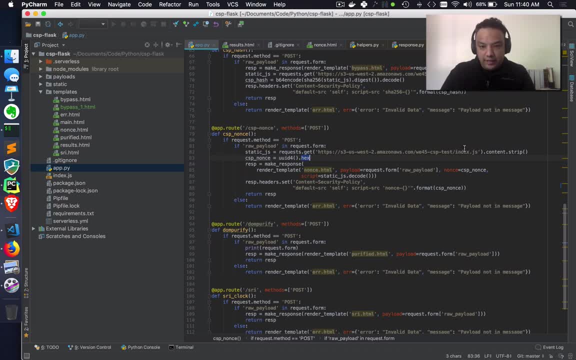 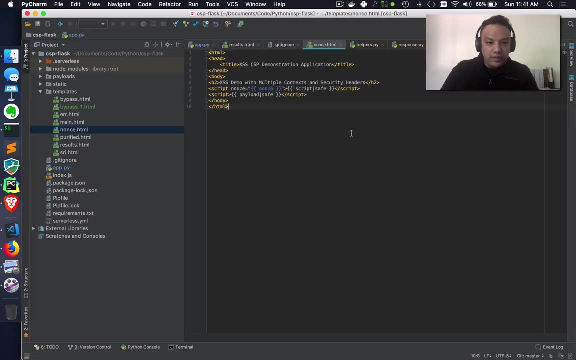 I'm going to do is I'm going to load the content of this particular JavaScript, and this JavaScript is going to be linked to the nonce. so if you look at the way it's going to work, you will see that I am loading the JavaScript on the front. 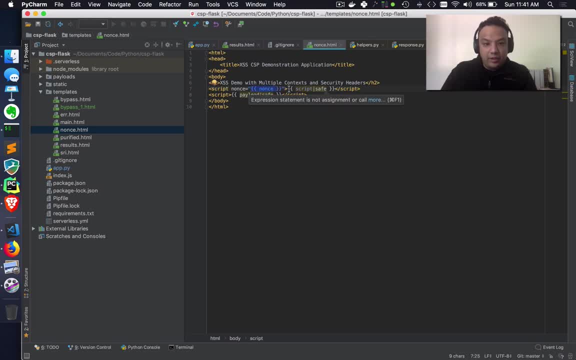 end with a particular nonce and I am also loading the JavaScript right and I'm also entering additional payload. so I'm entering an additional JavaScript payload and since this does not have a nonce, it should not load and the content security policy should enforce the violation. say that, look, I'm not allowing. 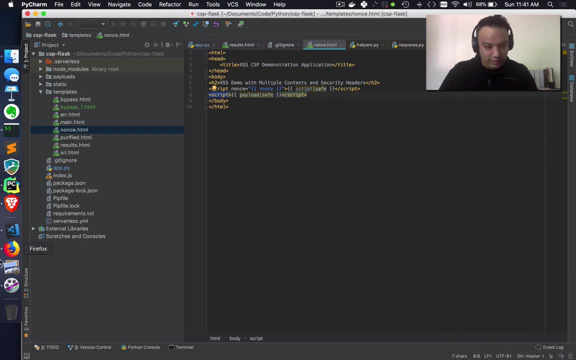 you to load this, simply because this particular script does not have a nonce. so in this case, what I'm doing is I'm using two JavaScript's. one is what is already being rendered by the nonce, and then this is something the attacker is trying to do: load his or her own JavaScript on your site, typically in. 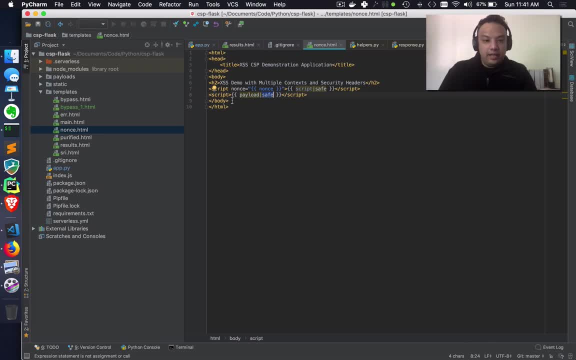 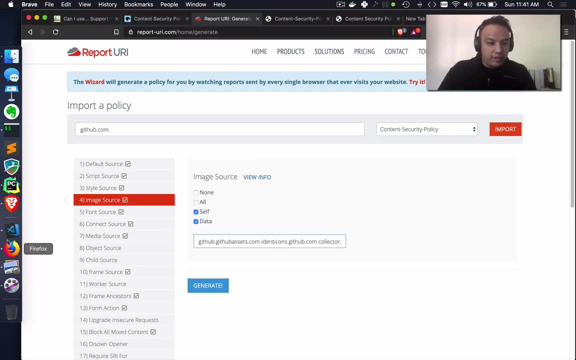 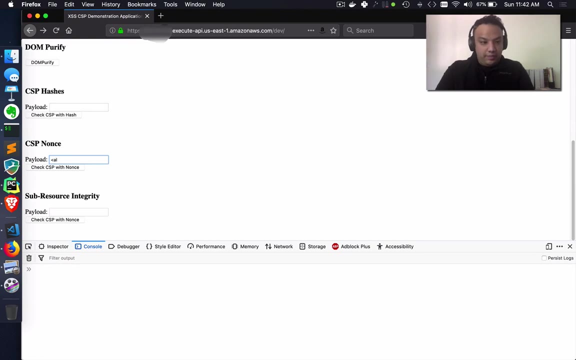 based on my existing content security policy, any script without a nonce should not load on that particular site. so let's look at how this works, right? so I'm going to go to go back to my demo site and I'm going to look at the nonce. so let's say I'm going to load script. 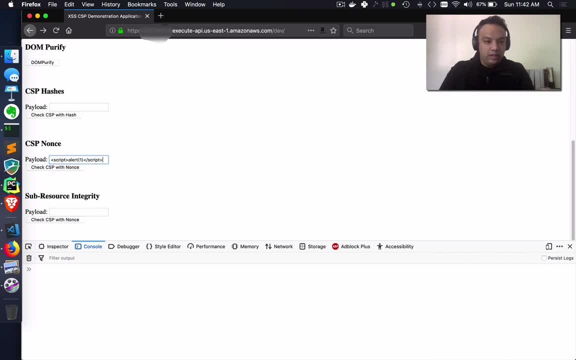 whatever, I'm going to just use something, script alert one, whatever. now, this should not load simply because I don't have a nonce for execution of this particular script. if I did, if this was linked to a particular nonce, I would load it. so let's look at how it works and you'll see that you should see the. 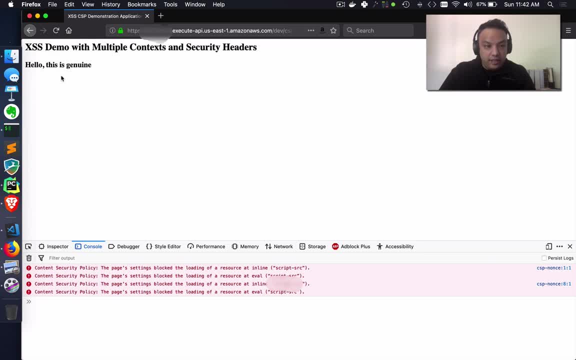 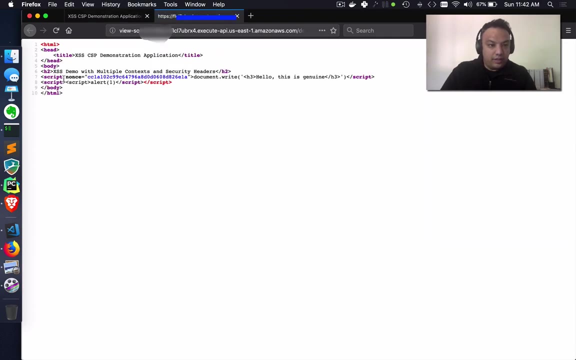 content security policy throwing up an error. so there are two things that I have happened here. the first thing is that the script with the nonce loaded. however, with the script without the nonce did not load. so let's look at the page source. so if you look at the page source, I have this particular script. 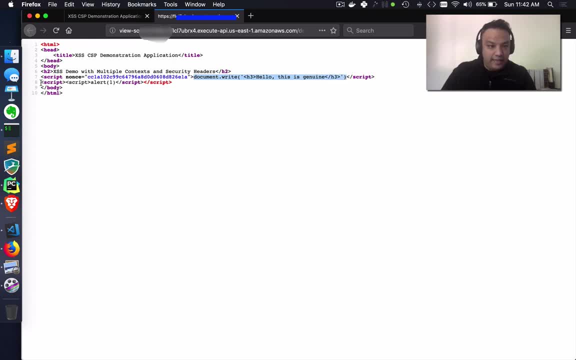 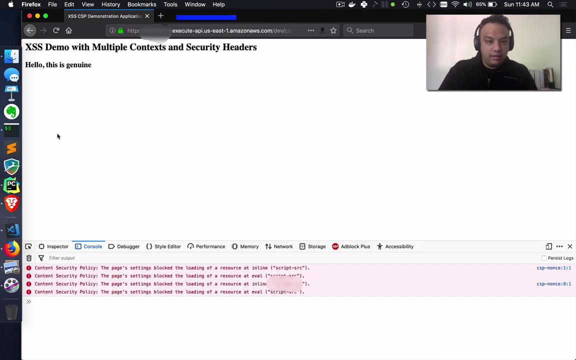 that loaded with the nonce and this script that loaded without the nonce right and this does not load simply because there was no nonce associated with it. however, let's say let's run the exercise again, so in this case I'm going to use alert hyphen one. 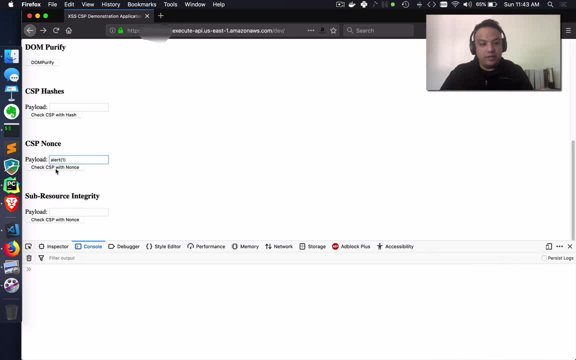 alert- sorry, alert- open parentheses, one close parentheses. so this is essentially going to to trigger a JavaScript alert now, since this is a script that I'm loading without a nonce right. so in this case, what I'm doing is I'm loading an existing script with a one-time token and I'm 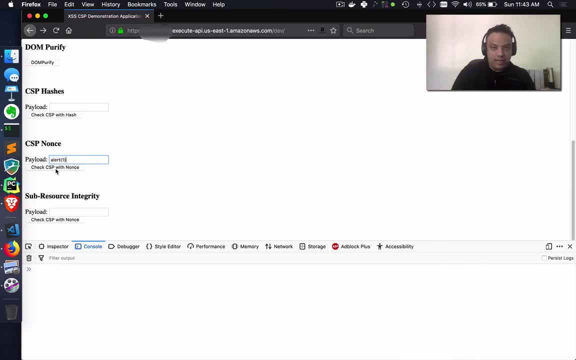 loading another script as an attacker without that token, right? so obviously, as an attacker, I can't guess the token. hopefully the token should not be guessable. well, that's another thing that you should keep in mind. the nonce should not be a guessable token. you should not make it 001, 002 or something that. 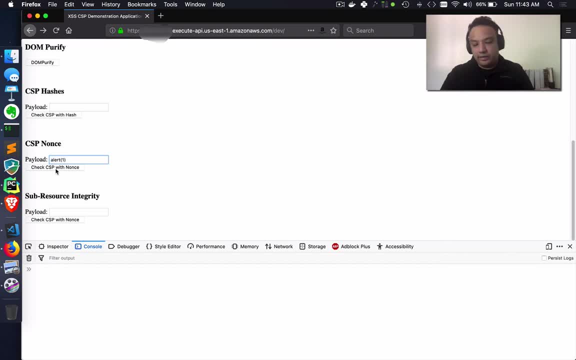 wrote something that is a random from a PRNG or a URandom or whatever it is. so in this case, what I'm doing is I'm loading this alert. typically, this should not work, because I don't have a nonce associated with it, and you will see soon. 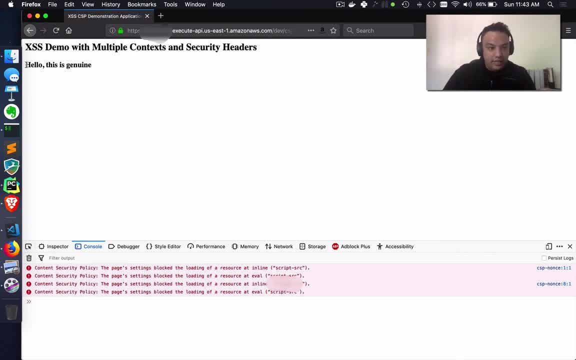 that does not work right. so the first thing that loads is the JavaScript that prints the documentwrite which says this is genuine. however, the alert did not load and let's look at what happened there. so if you look at the page source, you'll see why that happened. 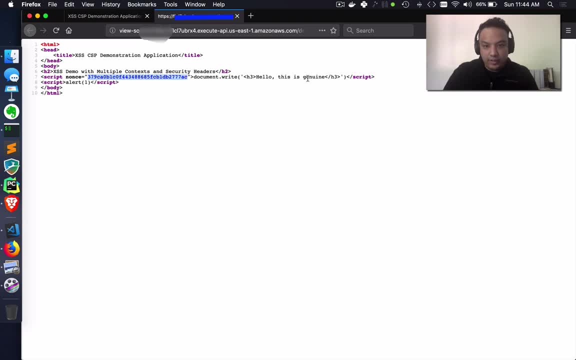 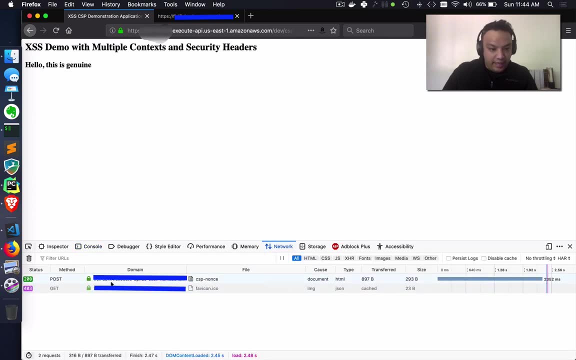 the first script that had the nonce which is the hello. this is genuine work. simply because it had a nonce associated with it, and if you look at my CSP header, you will see that anything with this particular nonce would work right. it would work because there is a specific nonce being applied to that particular. 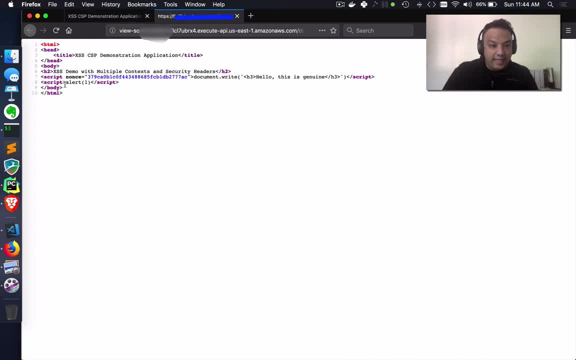 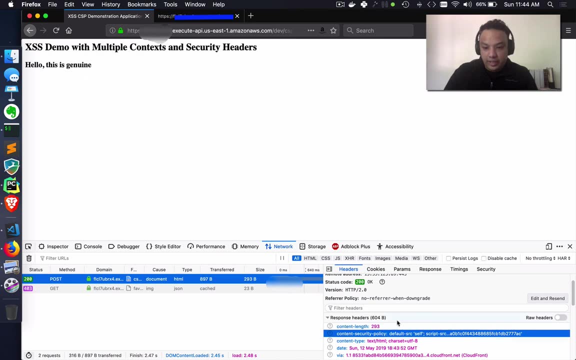 content security policy. however, the second script, which is supposed to load the alert function, did not load because there was no nonce associated with it. since the browser did not see that particular nonce, there was no real execution. that happened and the CSP policy essentially worked because the enforcement happened, the next type of CSP control I'm going to be talking. 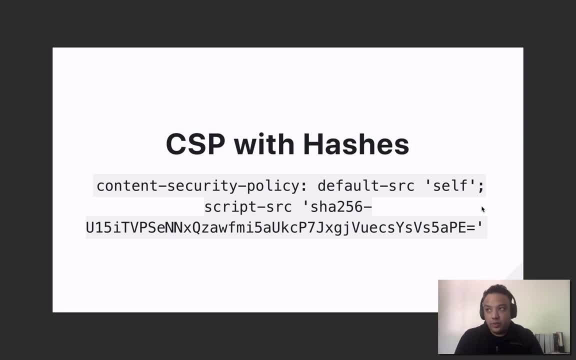 about is one with hashes right now. in this case, what we're doing is that we want to restrict the loading of JavaScript based on the hash value of that JavaScript, right? so in this case, what I'm going to do is- I'm going to give you an example- I have a JavaScript. 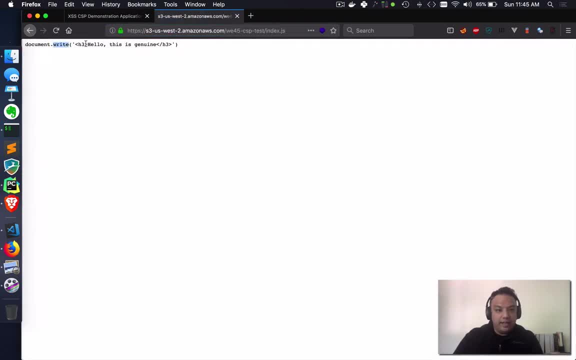 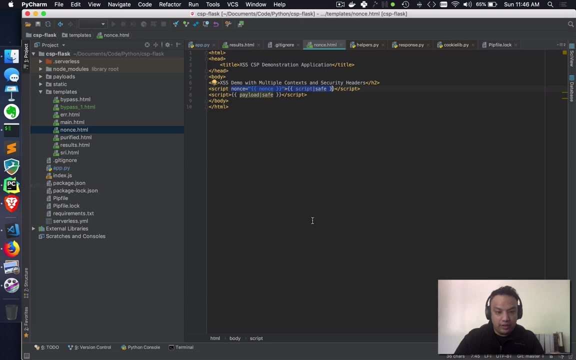 which is like: so right, documentwrite? hello, this is genuine. you've already seen this in the previous example. now I'm going to generate a hash value of this and use that to create my CSP. so in this case, what I'm doing- let's have a look at the code- is: 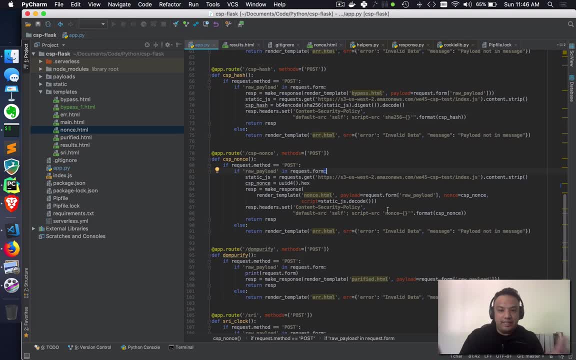 that I am loading. this is a contrived example. you would typically not need to do this. you can probably have all the hash values mapped out somewhere else and then loaded in HTML. so in this case, what I'm doing is I'm loading this indexjs file and I am hashing it with the SHA256 algorithm and base64. 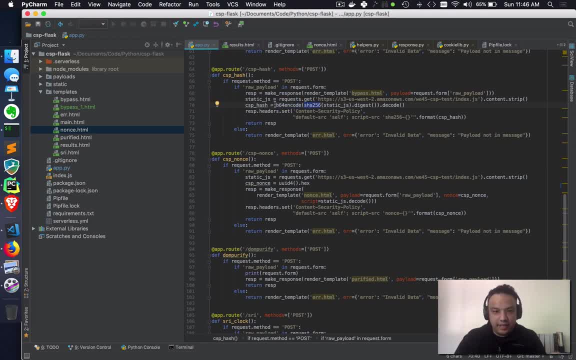 encoding it right. so I'm using SHA256 and then using base64 to base64 and code the code SHA-256 hash, right? so what I'm going to do is create my content security policy that says: default source: self script source: load only scripts if they have. 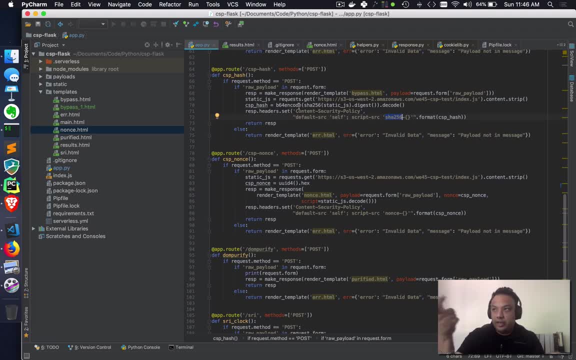 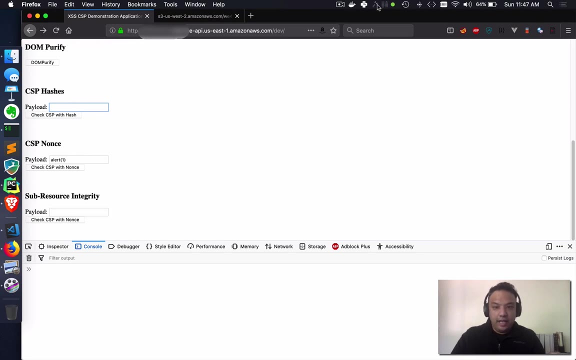 the SHA-256 hash. that matches with the SHA-256 hash of the JavaScript that you are loading, right? so let's look at how that works in our example application. so let's go back here and use the hashes. so let's say I am loading document dot. 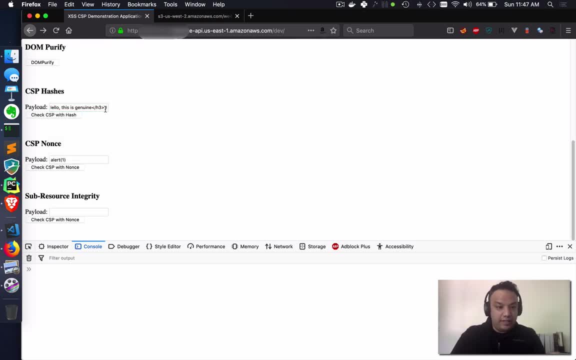 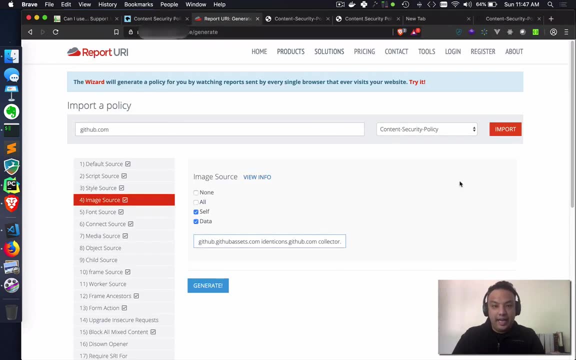 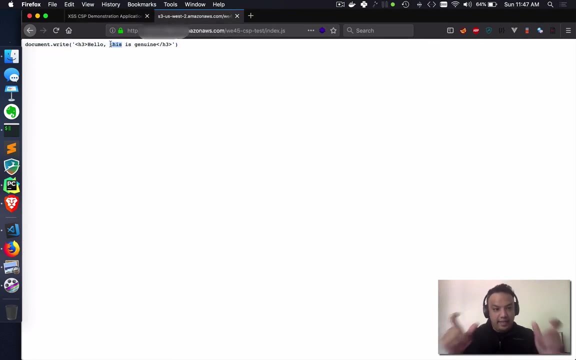 write. so let's say I'm loading this right now. this should work, simply because the hash of this particular value should match with the hash I have generated from the whitelisted JavaScript. so in this case, I have whitelisted this and exactly this particular JavaScript is the only thing that's going to load in. 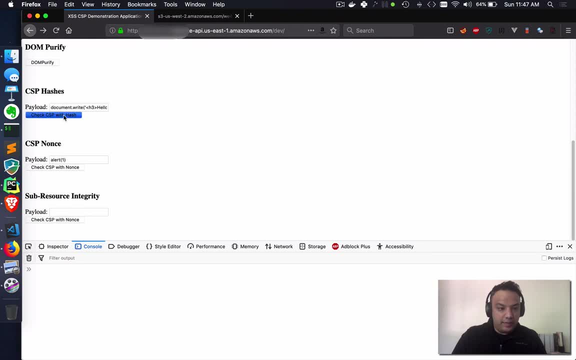 the application. so let's look at this and we see CSP with hash and it loads- and it should tell me that. so it loads the JavaScript. it says: hello, this is genuine, because now, since we have the hash, the JavaScript is loaded with said hash. right, that's the way it works. let's look at the. let's look at a different attack. 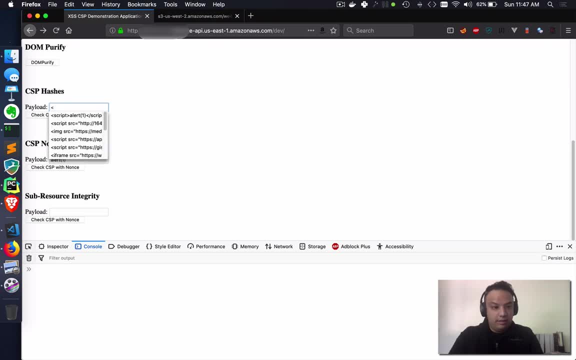 let's look at a different payload instead of this. let's just put in whatever script, alert something, dot IO, payloads, dot JS. now let's say let's take a different case or let's take another case. let's take alert document, dot domain, right, and hopefully it should not load and you can see that. 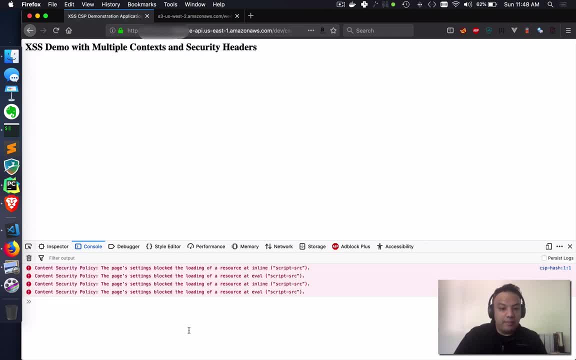 it does not load simply because it did not match that hash. it did not match the hash that we had provided for whitelisting that particular script. now this is complicated in that every single JavaScript that you have if you're using the hash approach, every single JavaScript needs to be the hash needs to.